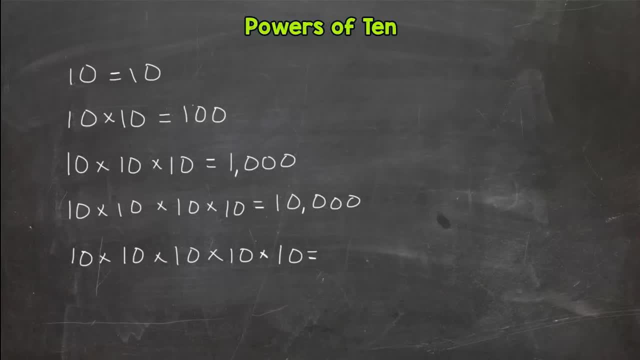 figure out what this is going to be right away, and hopefully you're thinking: 100 times, 10 times, 10 times 10.. So let's do one more. Let's do five 10s, 10 times 10 times, 10 times 10. 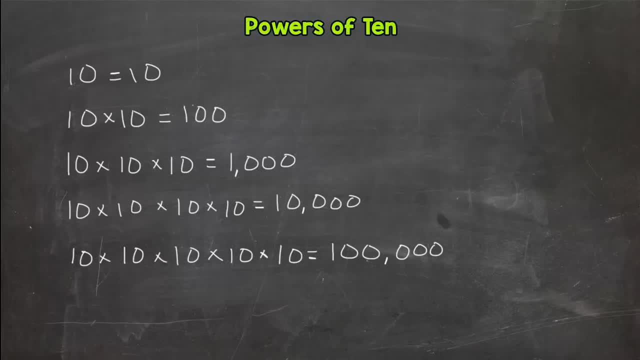 equals 100,000.. Now I could go on forever. I could put 10 times, 10 times 10, you know 100 times if I wanted to, But let's cut it off at five. This is plenty to recognize our pattern. And if you haven't, 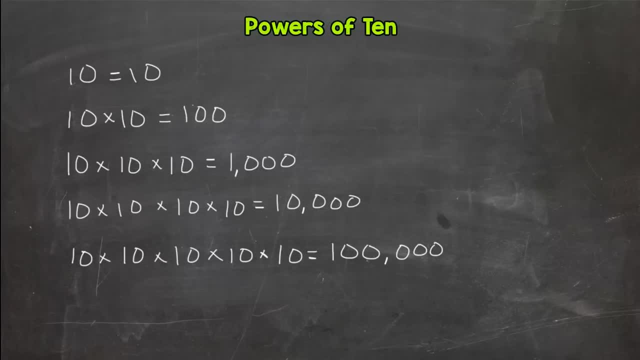 caught on yet. I would suggest taking a look at the amount of zeros in our number here. How many are there? One, two, three, four, five? How many tens did we multiply together here? One, two, three, four, five. It matches exactly. 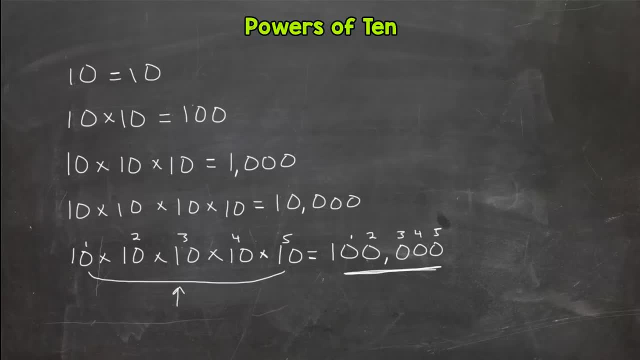 This right here, when we expand our tens out. we have five tens there. We can call that expanded form for our powers of ten. Expanded form: This right here, where we're writing out our numbers: ten, one hundred one thousand. ten thousand one hundred. 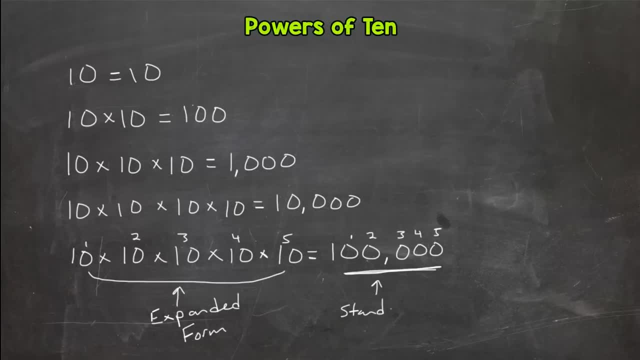 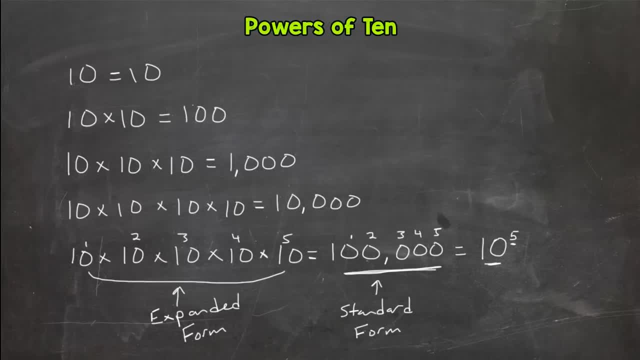 I think I got five there, So let's do this one. Sorry, let me back up. That is exponential form. Exponential form Because we use an exponent, And I'll talk a little bit about an exponent here in a second. 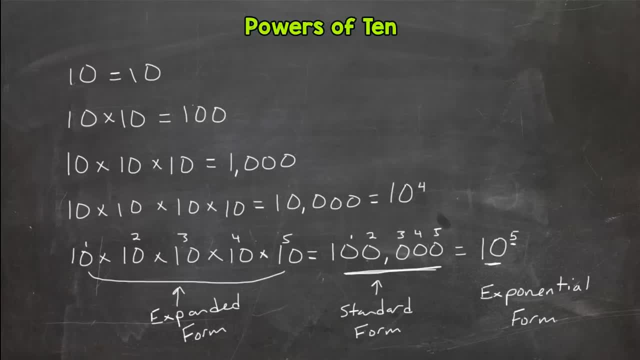 So this one we have, 10 to the fourth power, Four 10s, four 0s, exponent of four. It all matches. 10s are nice and easy to work with because these patterns work for 10s. This one we have, 10 to the power of three.